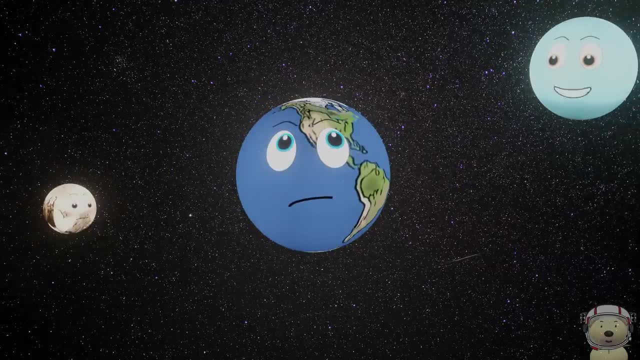 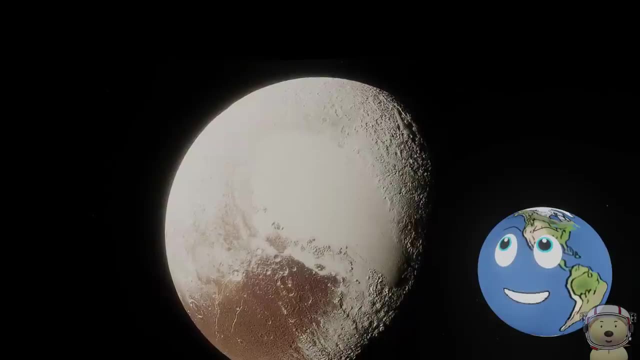 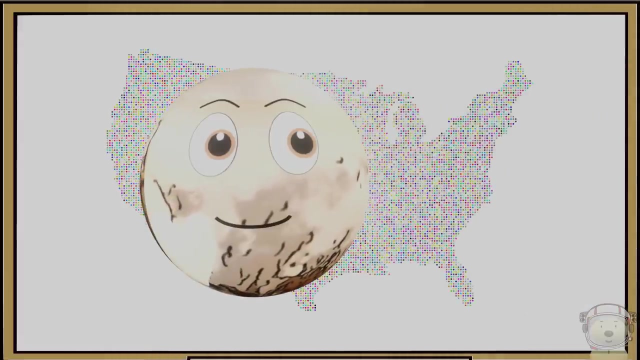 I'm still a planet, Not a planet. But do you realize just how small it is? It is actually only half as wide as the United States. Just look, Wow. That is like showing how small you are compared to me. Earth. 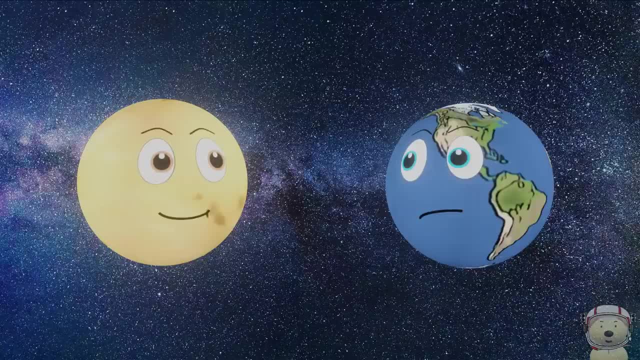 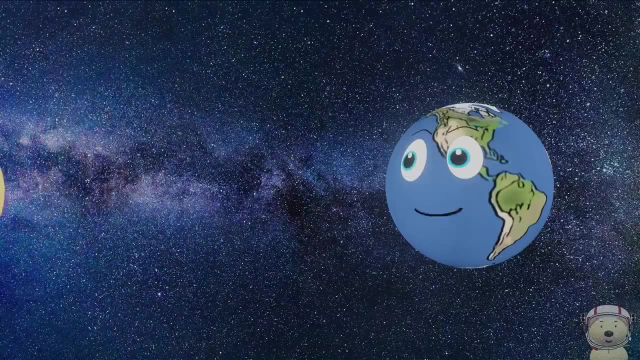 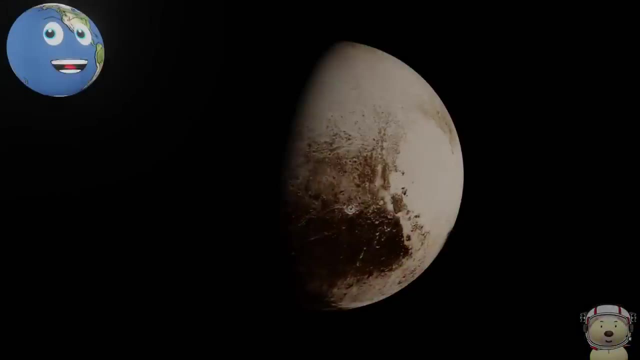 Yes, I kno. Wait a minute, Venus. I'm slightly bigger than you. Sure you are Earth, Sure you are. We're literally almost the same size. I know Earth, Sure. Pluto's diameter is only 2,370 kilometers. 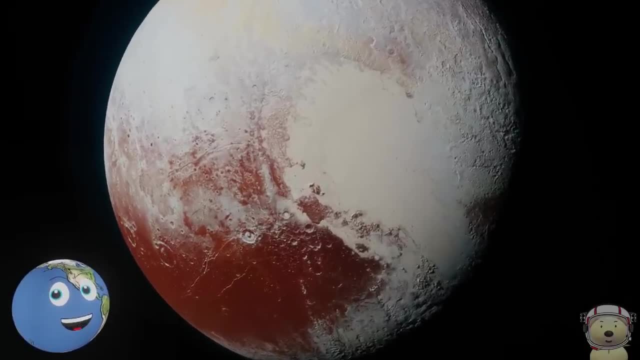 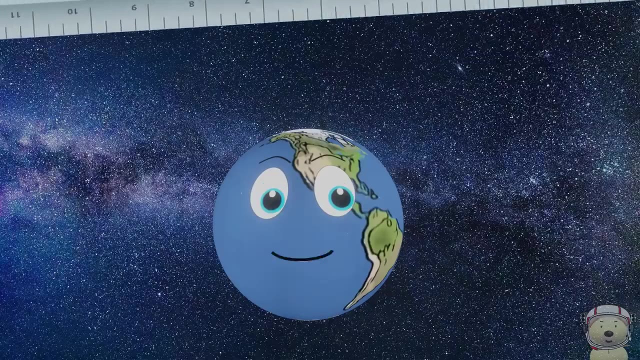 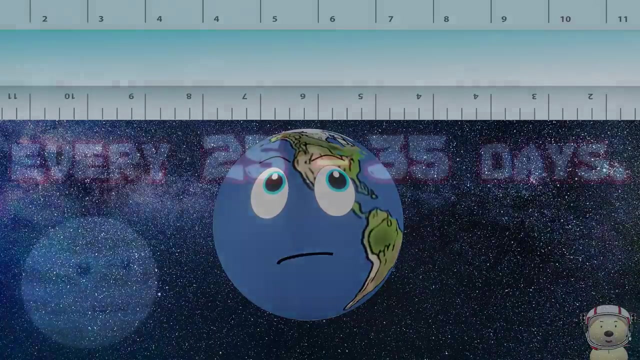 So in fact, it would be less wide than Australia. Just look at this. There you go On to the next fact: Venus, Neptune. The Sun makes a full rotation once every 25 to 35 days. Wait, wait, Jupiter. 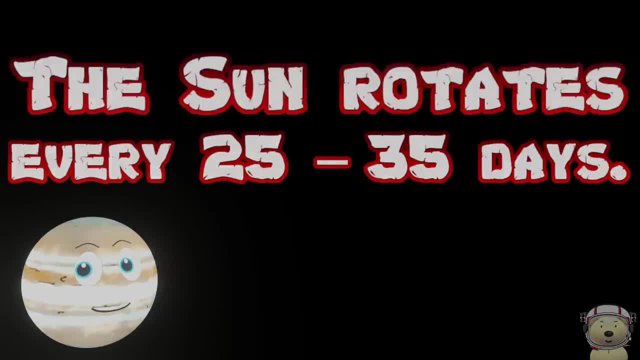 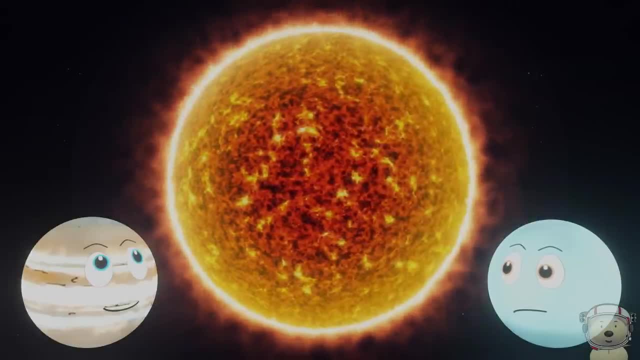 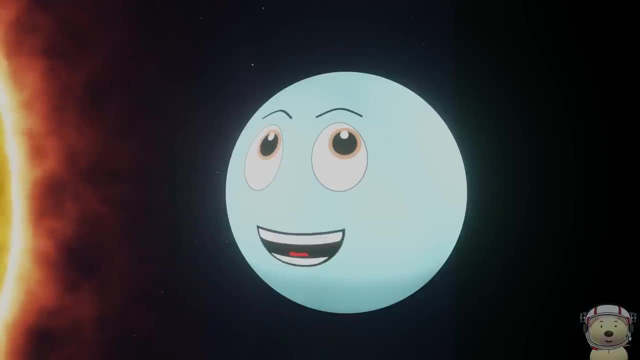 The Sun rotates. Yes, Uranus, The Sun does rotate. How can it rotate at different times? 25 to 35 days. That makes 25 to 35 days. That makes 25 to 35 days. That makes no sense. 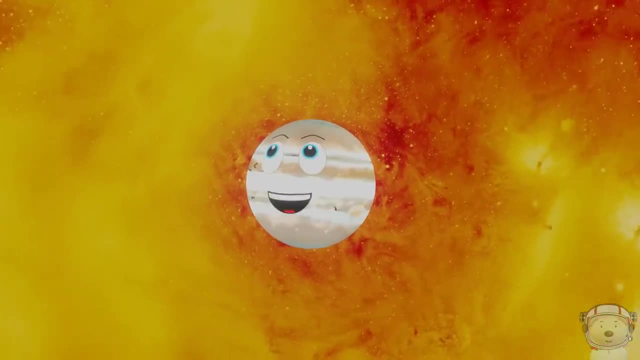 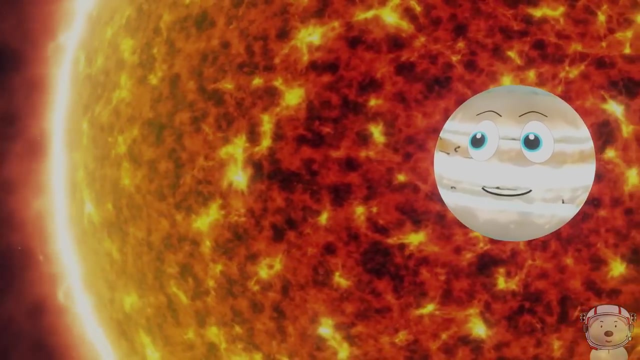 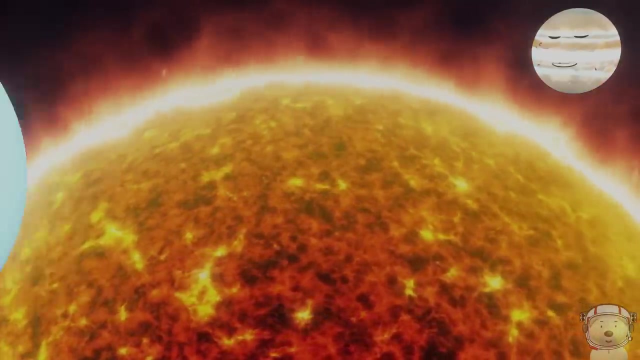 Well, on average, the Sun rotates on its axis once every 27 days, But its equator spins the fastest and takes about 24 days to rotate, Whereas it takes more than 30 days to rotate at its poles. Wait, wait. 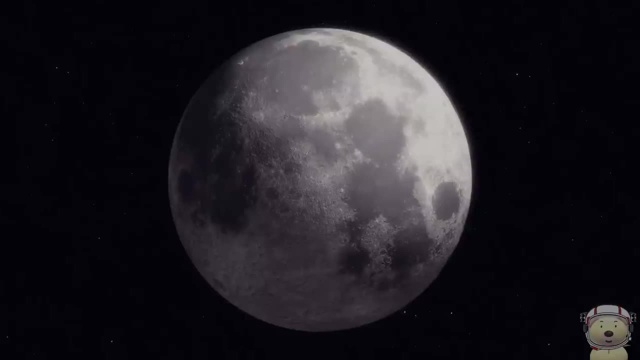 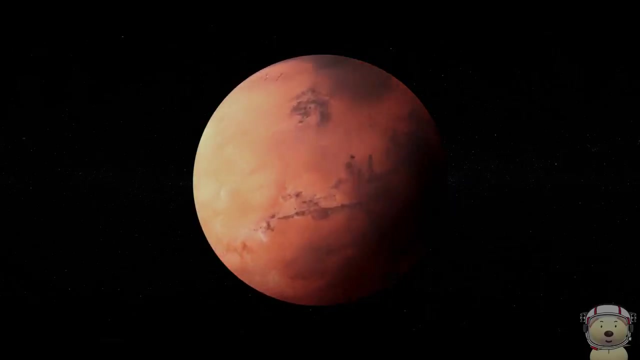 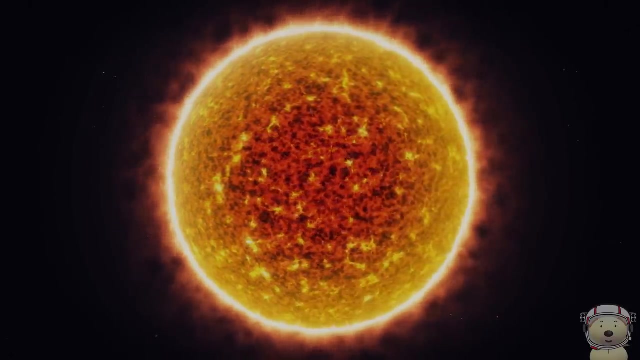 You're telling me that we planets have moons rotating on their axes while they orbit around us. Well, we planets rotate on our axes while we orbit the Sun That is rotating on its own axes While the Sun orbits us around the center of the Milky Way galaxy. 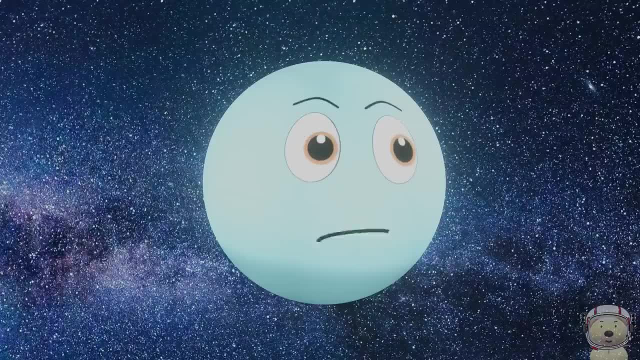 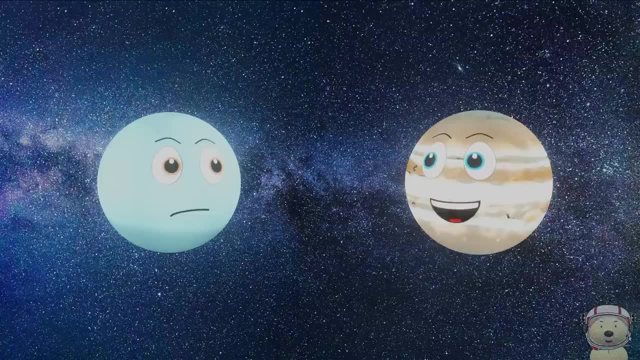 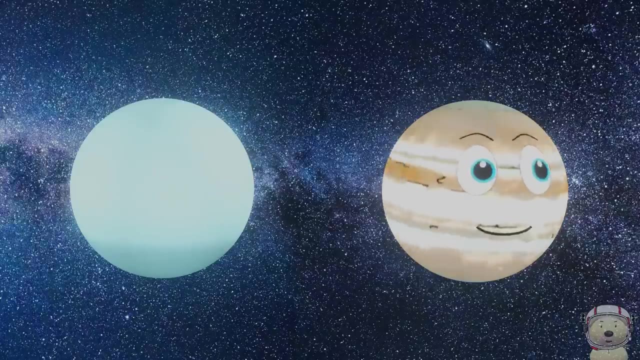 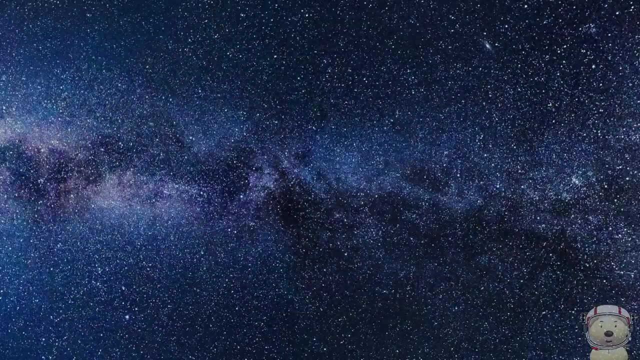 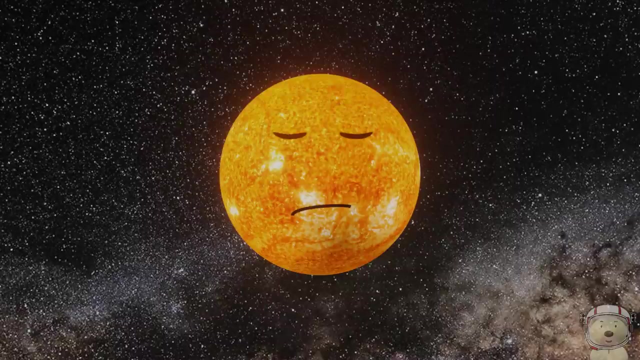 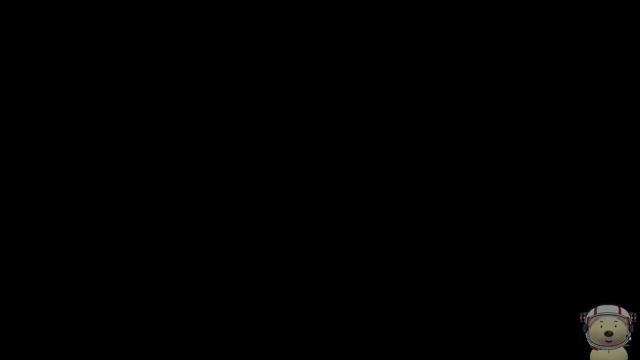 Yes, My head hurts thinking about it. I am the fastest rotating planet in the solar system. See if you can rotate as fast as me. Uranus, Ready Go, Woo-hoo, Whoa, All right. Whoa, The whole of Mars is as cold as the South Pole. 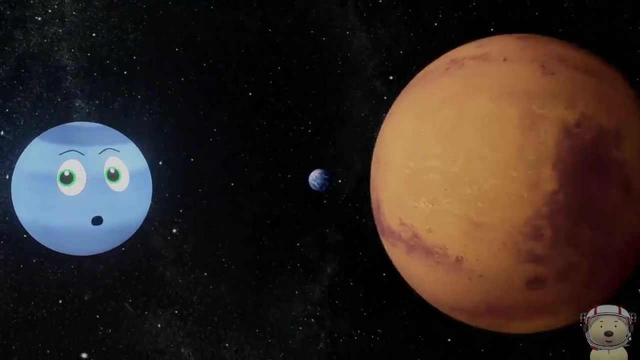 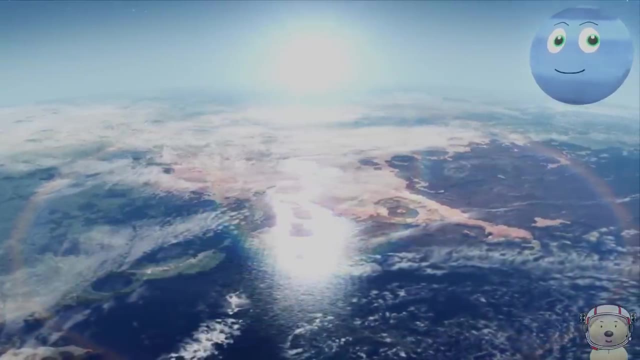 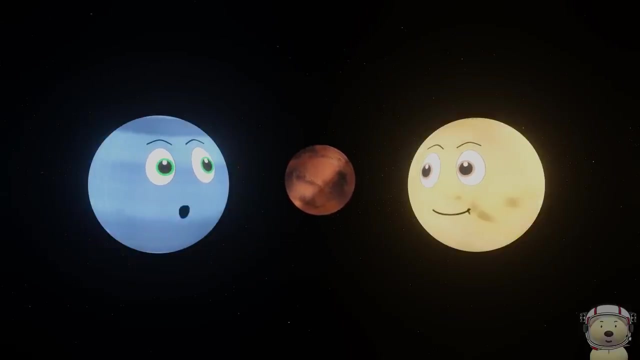 Now we all know that Mars is one of the closest planets to the Earth, But it is that much further from the Sun that it makes the whole planet colder than the South Pole. How cold does Mars get, then? Well, on average, about minus 81 degrees Fahrenheit. 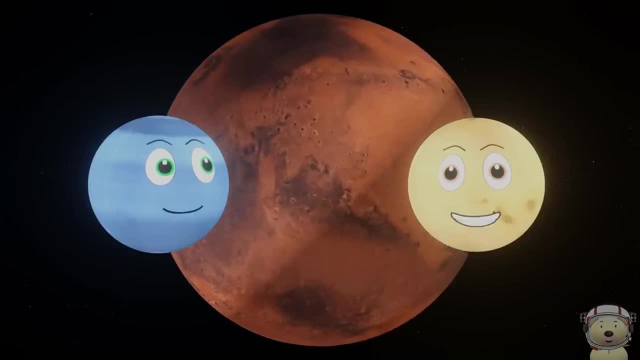 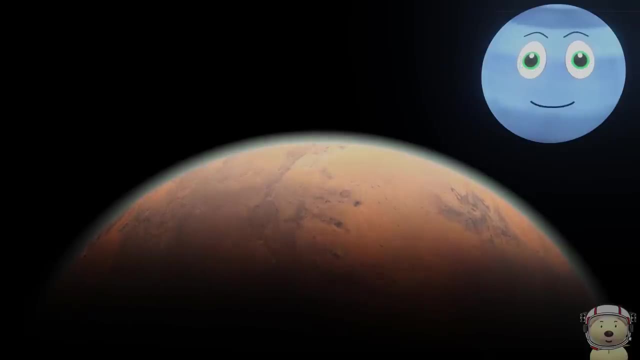 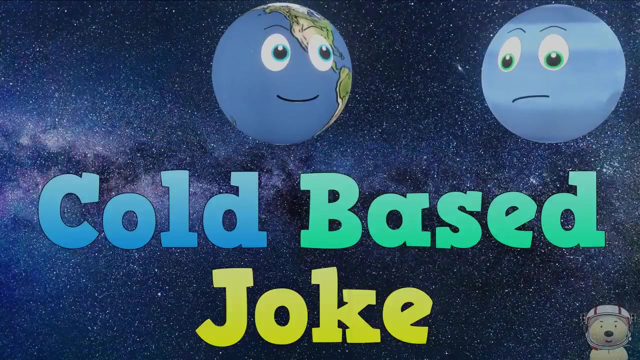 Wow, I wouldn't ask too long a mass. No, Although it looks red and hot, it is in fact very cold. Hey Neptune, I have a cold-faced joke for you. Oh no, Not this Knock knock. 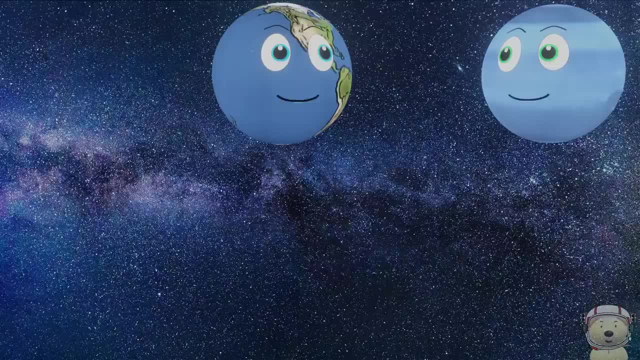 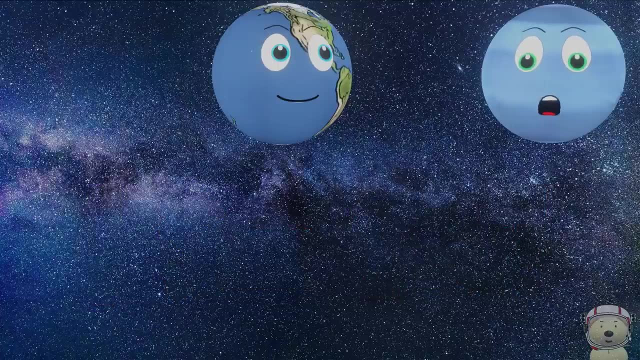 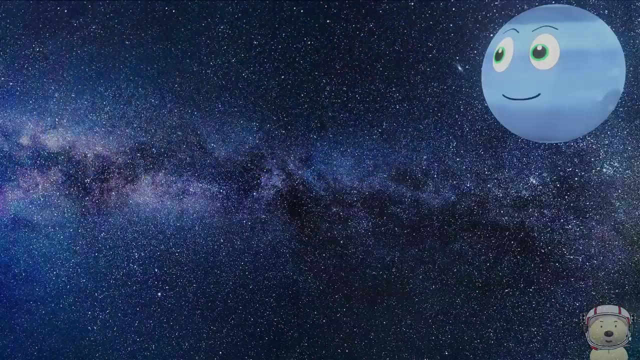 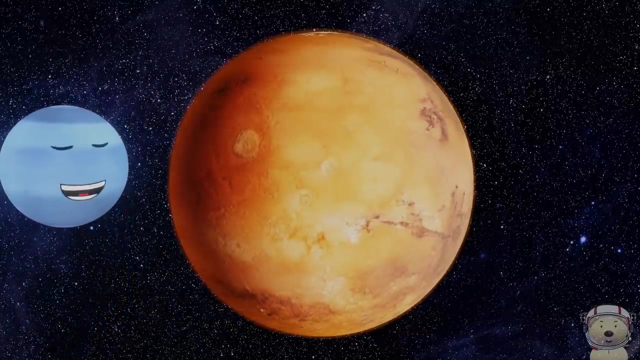 Who's there? Icy Icy, who Icy you. Somebody get him out of here. Come with me, please, sir. As well as being further from the Sun than Earth, its atmosphere is very thin, so it keeps little heat in. 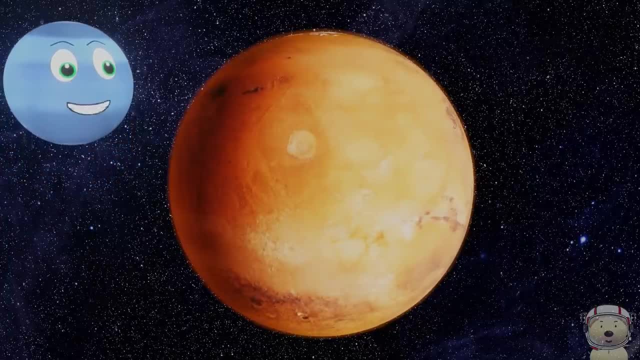 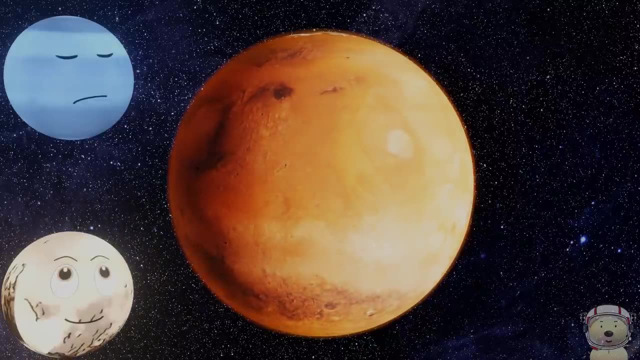 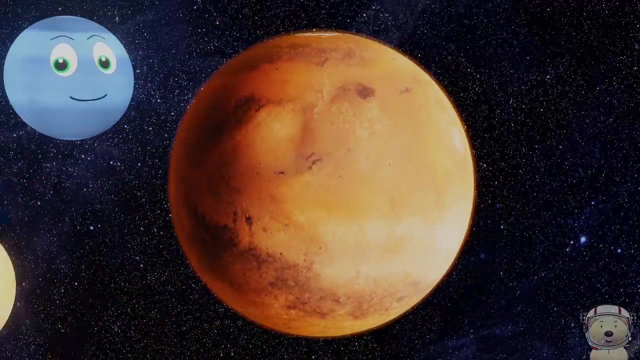 At Mars's equator, temperatures can reach 20 degrees Celsius, But overall, Mars is a very cold planet. Not as cold a planet as me, though, Pluto, you are not a planet. I'll take care of this. There you go, dudes.